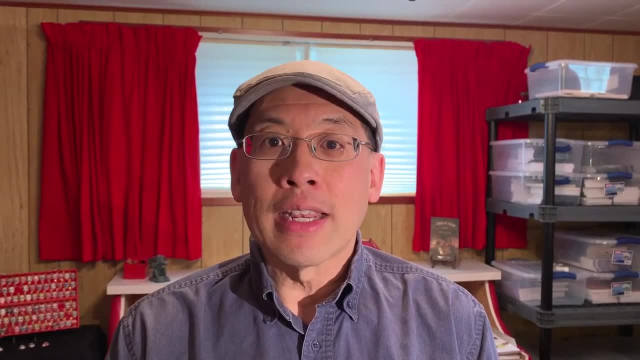 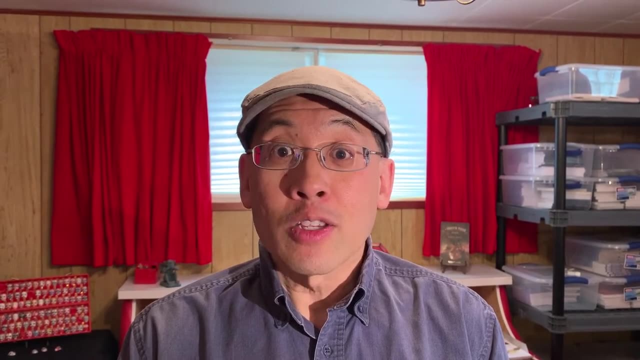 writing and share practical tips that you can use to get your kids excited about writing. In this video, I'm going to focus on story prompts, story starters that will get kids working on their own stories. In fact, I've got three story prompts. 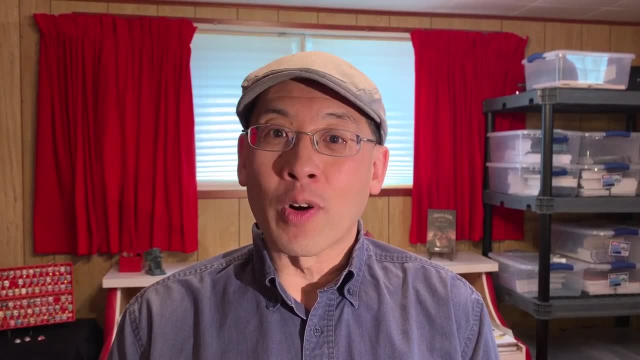 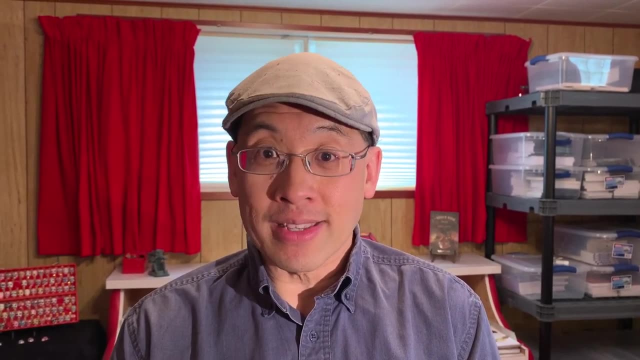 to encourage students to start writing- one for younger students, one for middle students and one for older students. But before I go down that road, I'm going to share with you a story of how I was motivated to become a writer myself. 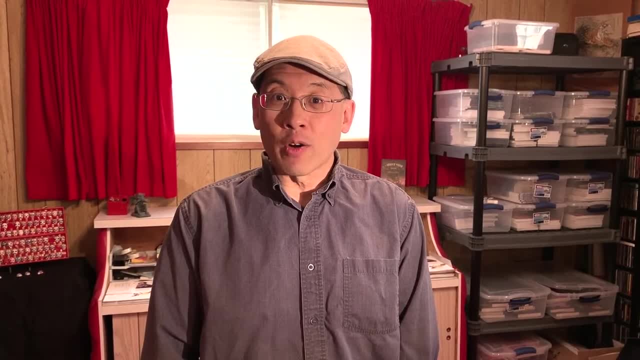 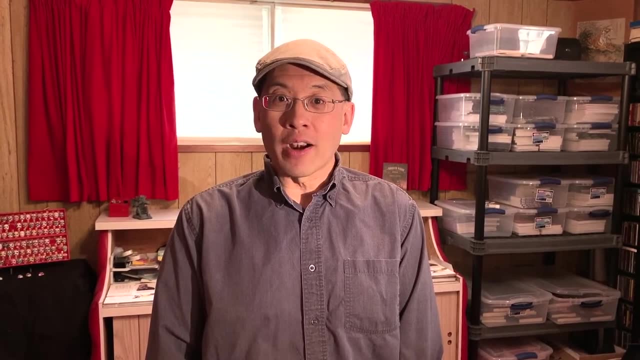 I had a language arts teacher named Mr Nigro and he was the best teacher I ever had. He gave our class a homework assignment. He said: imagine you've won the lottery and you have a million dollars at your disposal You can use. 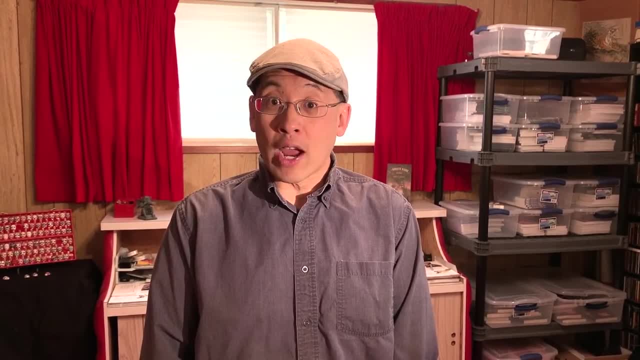 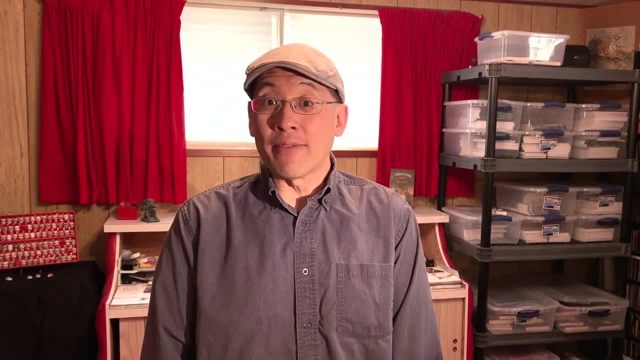 that money and buy anything you want. I just want you to describe how you'd use that money to redecorate your bedroom. Now, I was a lazy teenager, so my idea of a dream bedroom was to have a bed I never had to get out of, to do all the 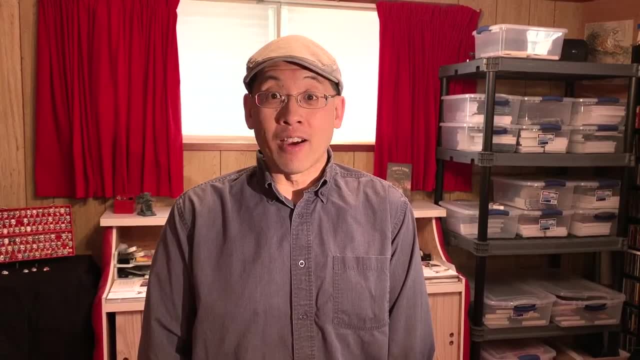 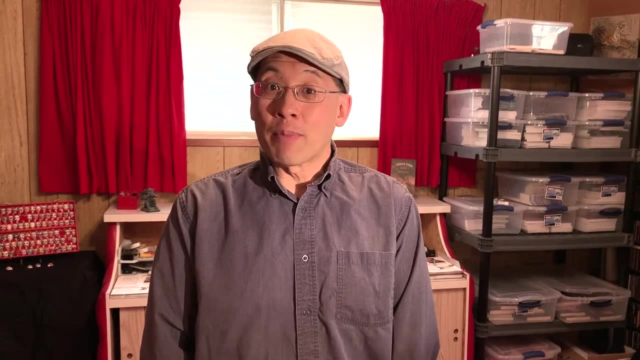 things I wanted to do. So I put my bed on an elevator. Top level is where I slept. There was a skylight overhead so I could sleep under the stars. Right beside the bed there was an elevator button on the nightstand. I pushed it and the bed would. 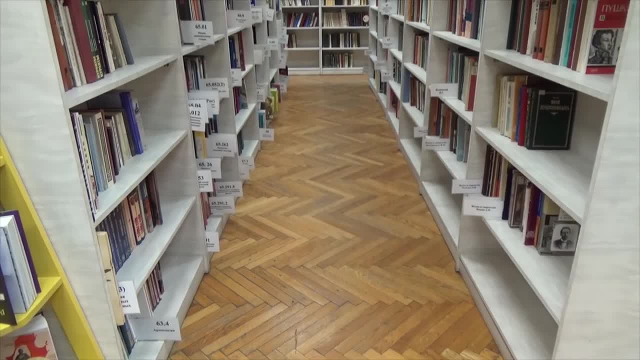 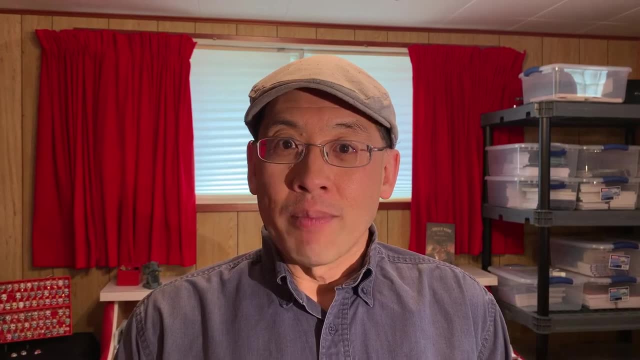 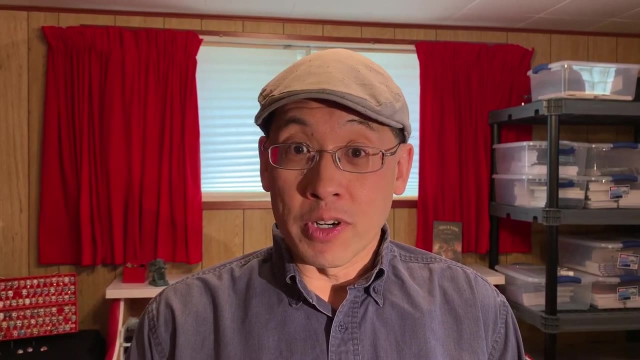 lower to a library with all the books I wanted to read. Next level had a big-screen TV, all the movies I wanted to watch. Underneath that there was a kitchen and a bathroom, But the kitchen had an automatic fast-food dispenser so I could get a Big Mac, KFC and a slice of pizza with the push of. 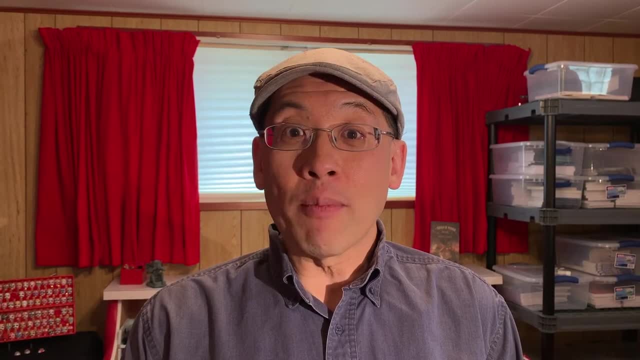 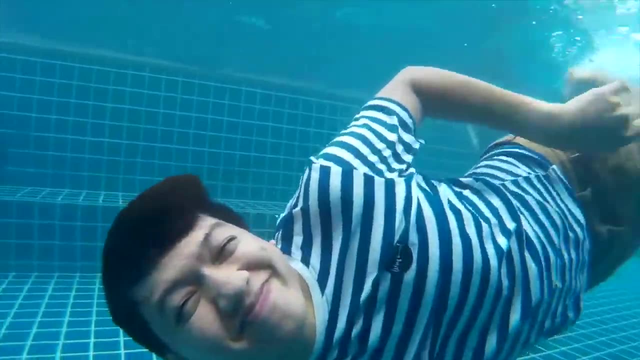 three buttons. Underneath the kitchen there was a video game arcade with every game system in the world And below that best level of all, it had an indoor swimming pool. I remember I handed in that assignment and Mr Nigro gave it. 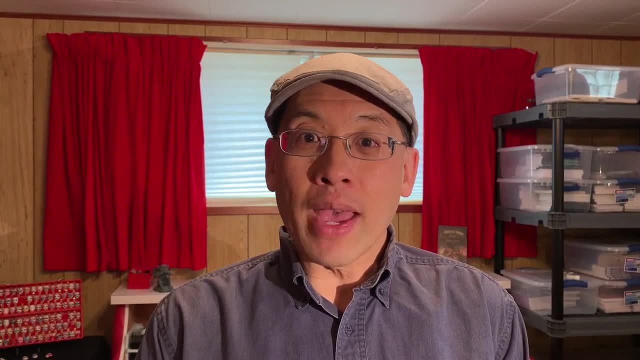 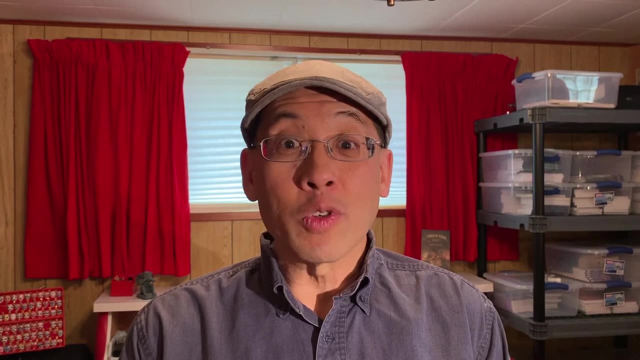 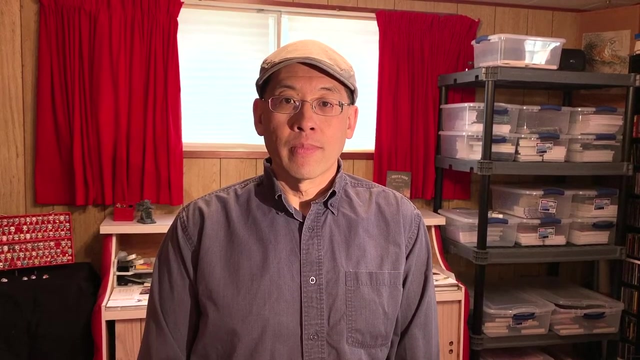 back to me a couple of weeks later and he said: Marty, you've got a great imagination, you should become a writer. Well, that's what I did, and now I'm gonna share with you those story prompts. This story prompt is a tribute to my language arts teacher, Mr Nigro. I want 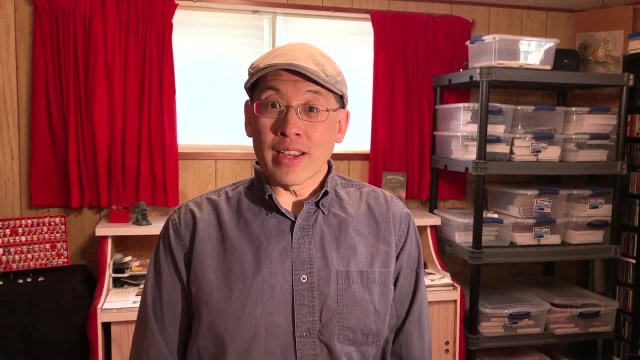 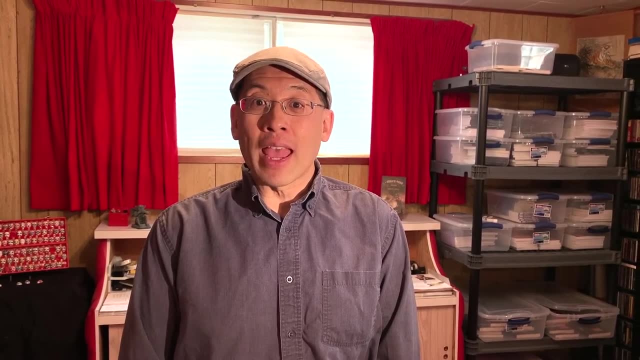 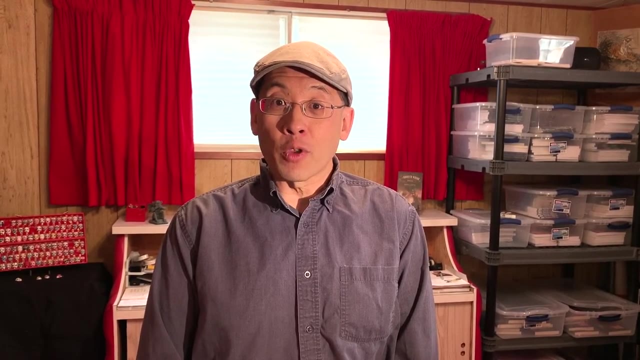 you to ask your students to imagine that they've won the lottery and they have a million dollars at their disposal. They can spend that money on anything they want, but they have to describe how they use that money: to buy things to redecorate or renovate their bedroom. The 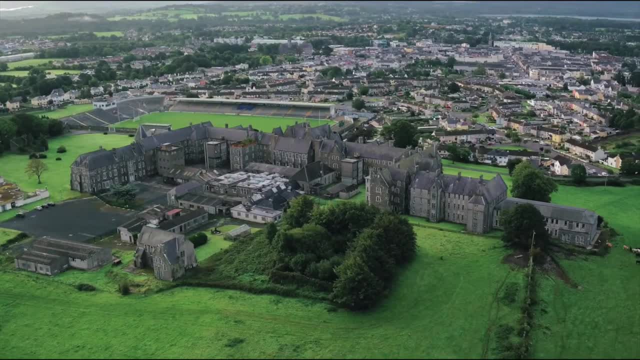 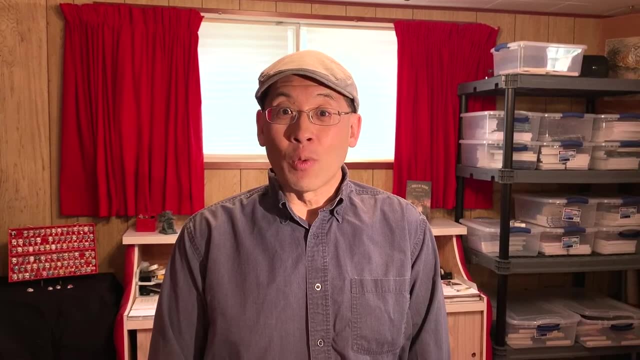 sky's the limit. They can buy anything they want, but they have to be specific about how they would redecorate or renovate their bedroom. Let's see what kind of amazing stories they'll come up with when they have a million dollars and they can do anything to their bedroom. 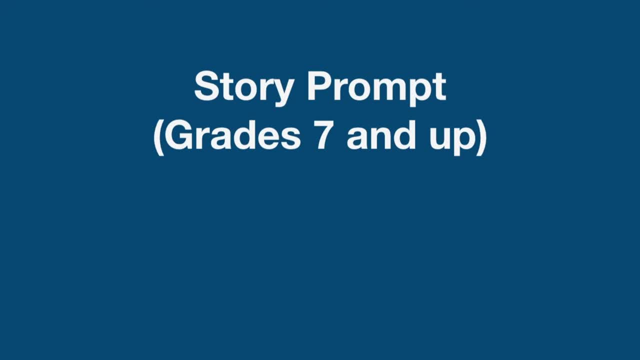 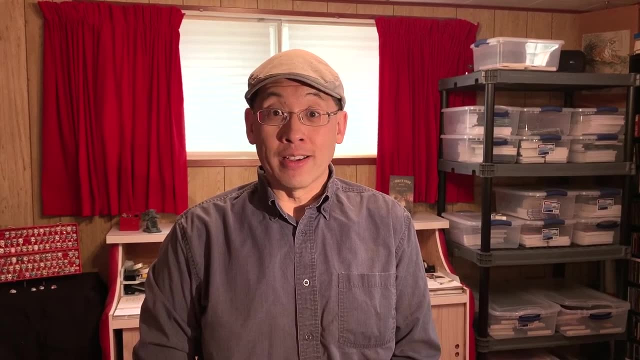 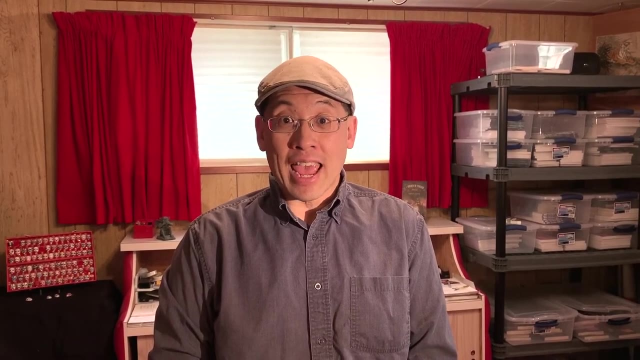 For this story prompt, I'm gonna rip a page out of the improv book. In improvisation there is a classic rule that every improviser follows, and that rule is yes, and That's where you take an offer and you add to it. and in this case, 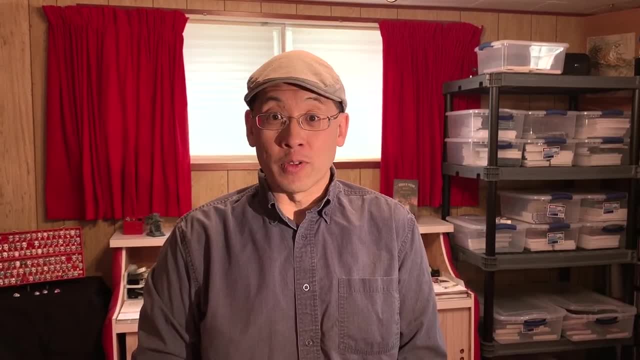 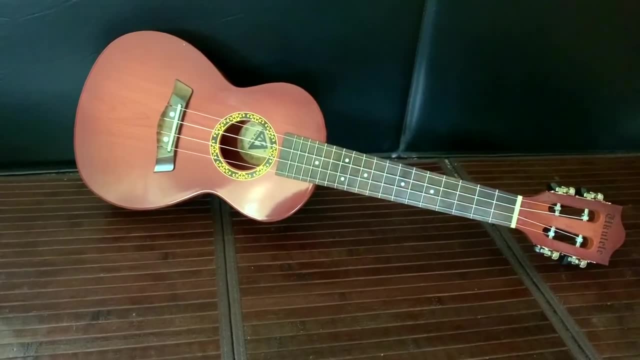 I'm going to have three offers for the students. There are three objects that they will have to incorporate into their story at some point. Doesn't have to be the beginning of the story, could be the middle, could be the end, but three. 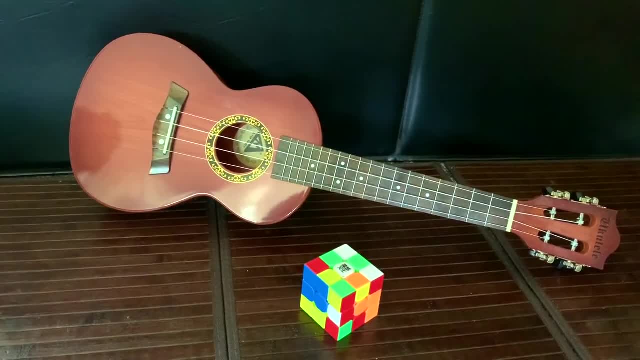 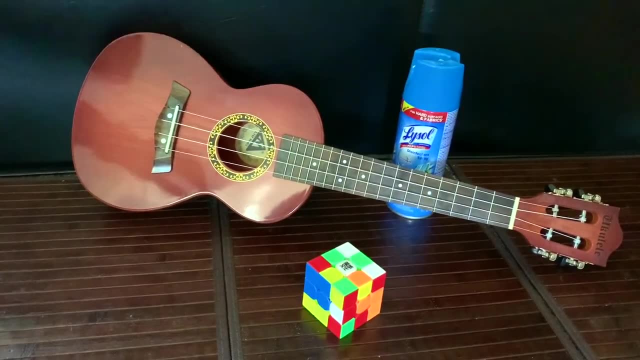 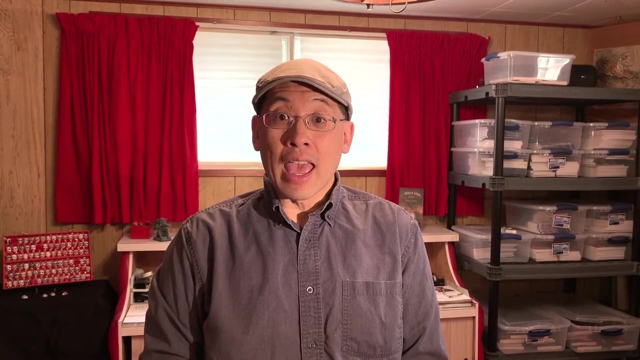 objects that they have to play with. In fact, think about this. Challenge them to think of these three objects as objects that they need to use to get out of an escape room. How are they going to use a Rubik's Cube, a ukulele and a can of? Lysol to be able to escape from their bedroom? How are they going to use a Rubik's Cube, a ukulele and a can of Lysol to be able to escape from their bedroom? How are they going to use a Rubik's Cube, a ukulele and a can of Lysol to be able to escape from their bedroom? 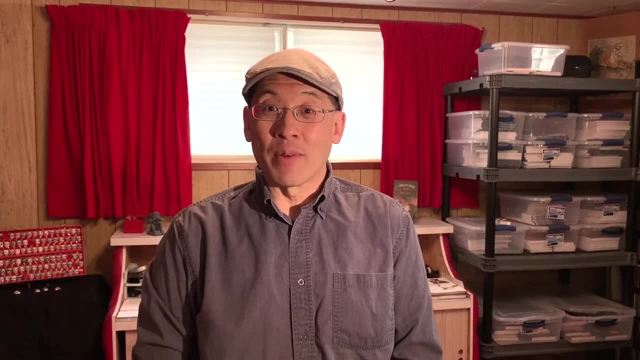 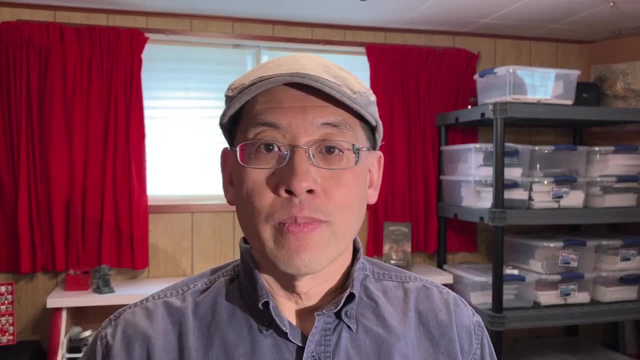 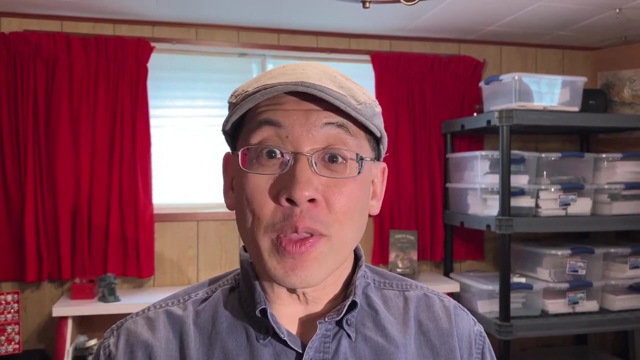 Let's see what kind of stories they come up with. This story prompt is for younger kids. One of the challenges of getting younger kids to come up with stories is they're still trying to figure out the mechanics of writing. So let's focus on getting them to tell stories, and it's always 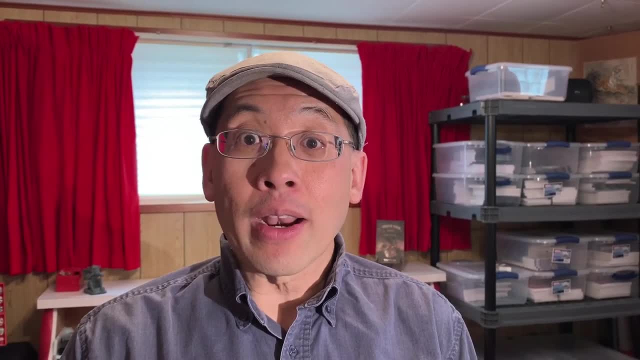 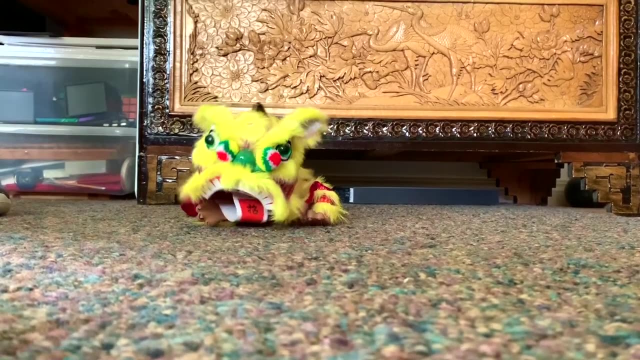 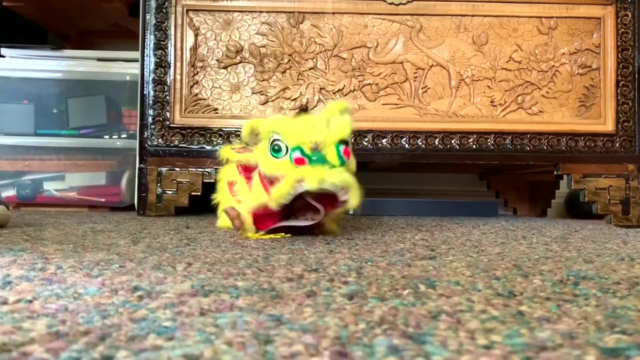 great to make something personal for the little kids. So what I am going to offer up is their stuffy story prompt. My ideas are: I am going to put my favorite character star and I choose either their favorite toy or their favorite stuffy and ourни grandes, du'ffi's or toys. I want them to pick their favorite toy, their